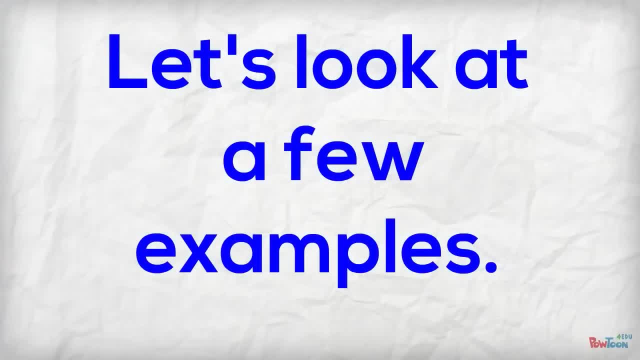 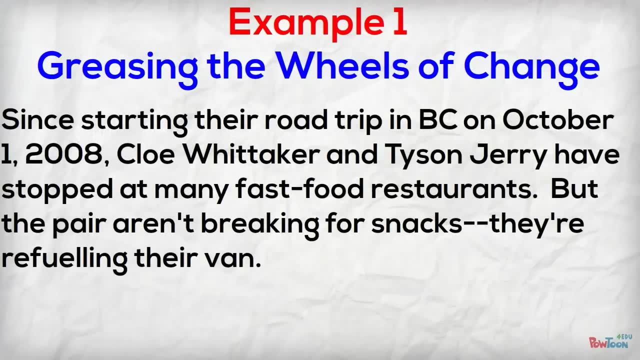 Let's look at a few examples. Example 1. Greasing the wheels of change. Since starting their road trip in BC on October 1, 2008,, Chloe Whitaker and Tyson Jerry have stopped at many fast food restaurants. 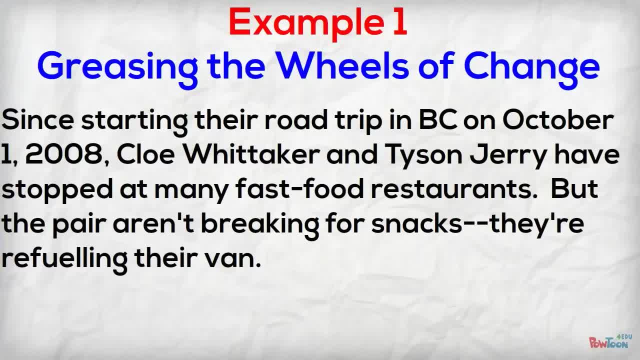 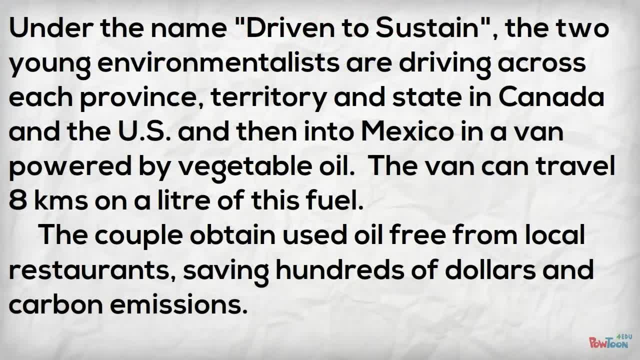 But the pair aren't breaking for snacks. They're refueling their van Under the name Driven to Sustain. the two young environmentalists are driving across each province, territory and state in Canada and the US and then into Mexico in a van powered by vegetable oil. 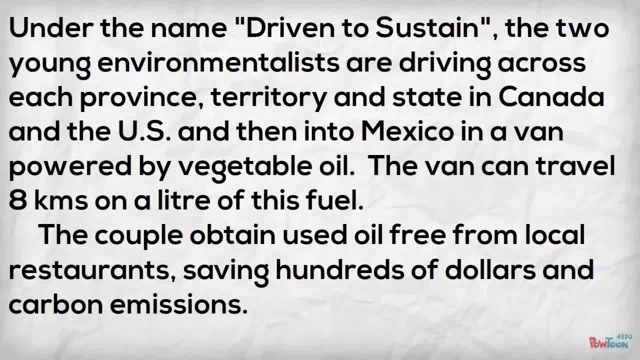 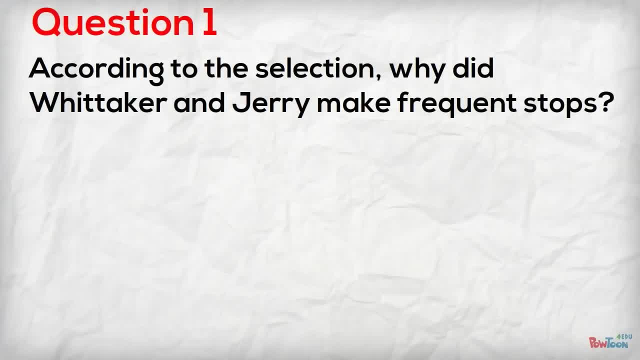 The van can travel 8 km on a litre of this fuel. The couple obtained used free oil from local restaurants, saving hundreds of dollars and carbon emissions. Question 1. According to the selection, why did Whitaker and Jerry make frequent stops? 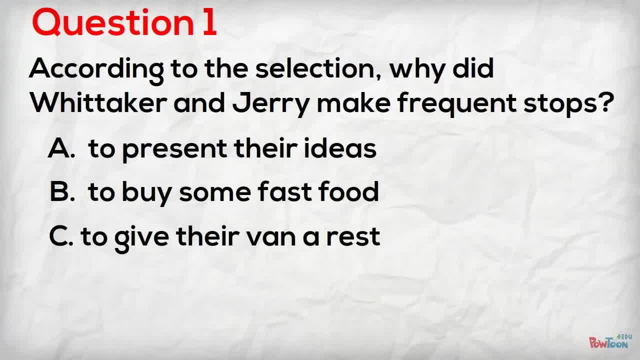 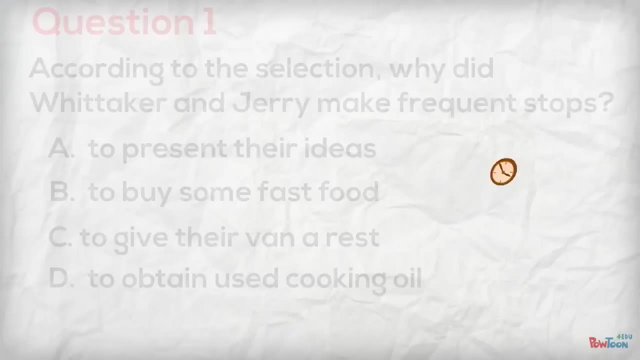 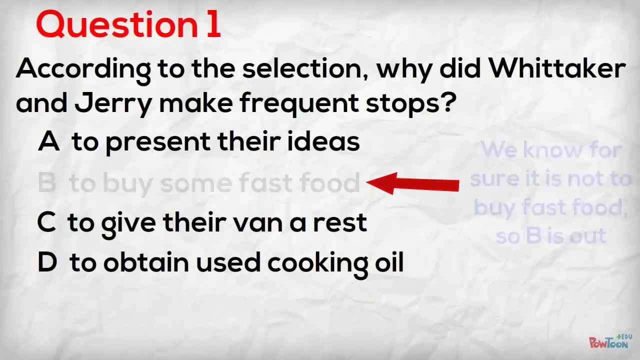 A To present their ideas. B- To buy some fast food. C- To give their van a rest. D- To obtain used cooking oil. We know for sure it is not to buy fast food, So B is out. It says nothing about presenting ideas or giving their van a rest. 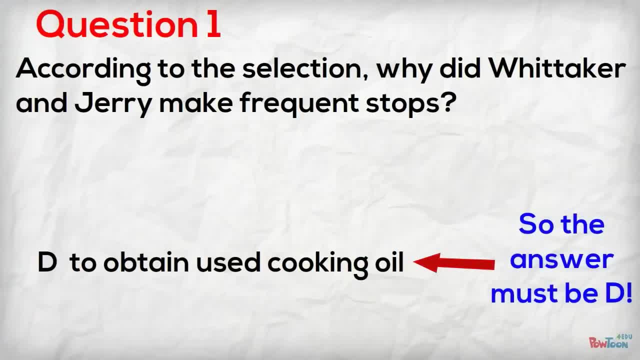 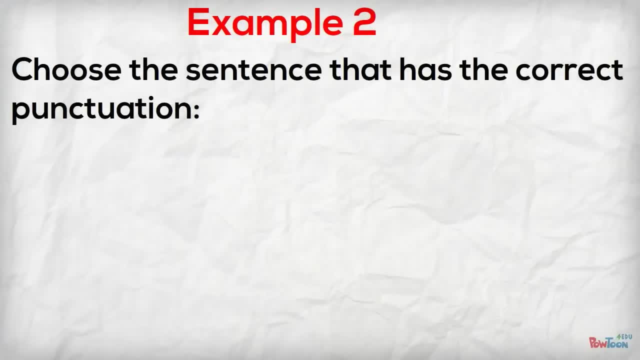 So A and C are out, So the answer must be D. Choose the sentence that has the correct punctuation. A- I like Ted's car because it's red and isn't noisy. B- I like Ted's car because it's red and isn't noisy. 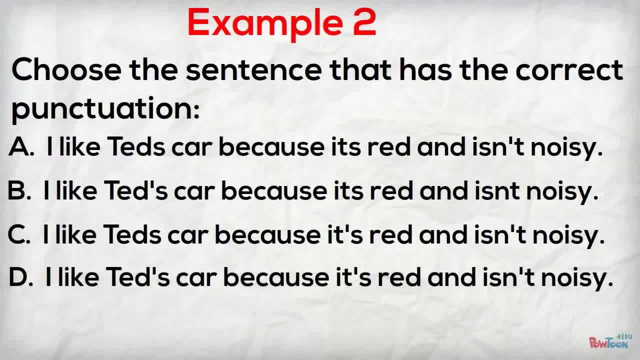 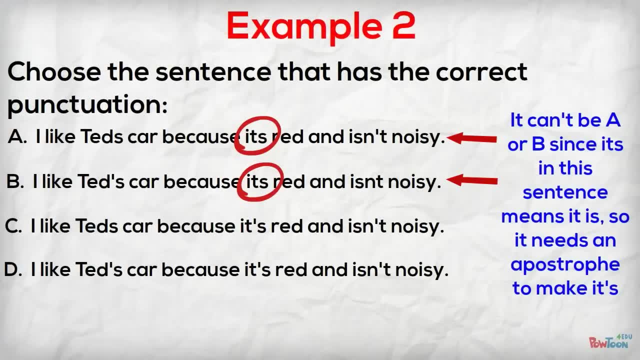 C- I like Ted's car because it's red and isn't noisy. D- I like Ted's car because it's red and isn't noisy. Or D- I like Ted's car because it's red and isn't noisy. It can't be A or B, since it's in this sentence means it is.